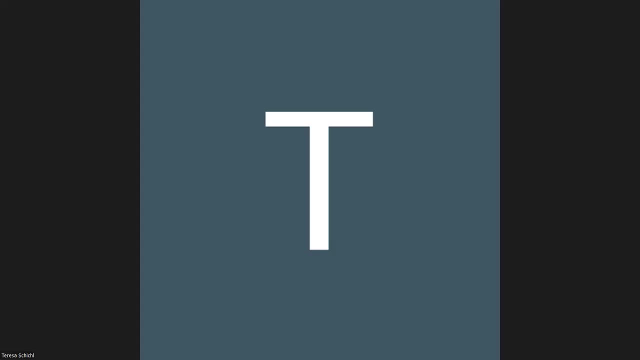 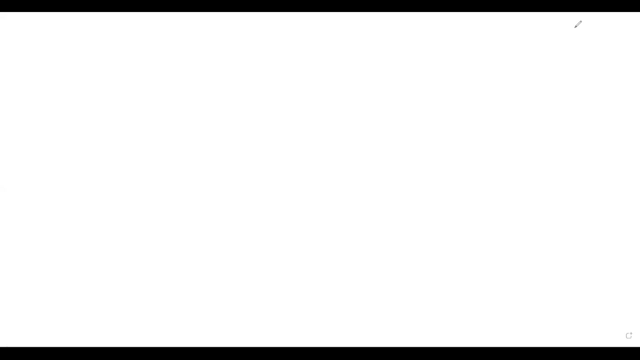 Okay, so now let's go to our whiteboards here and all right, so let's take a look. This is a very, very fun probability problem here. Okay, so the first thing here. let's see here: I have r-boxes here, right? So this is the r-box here. 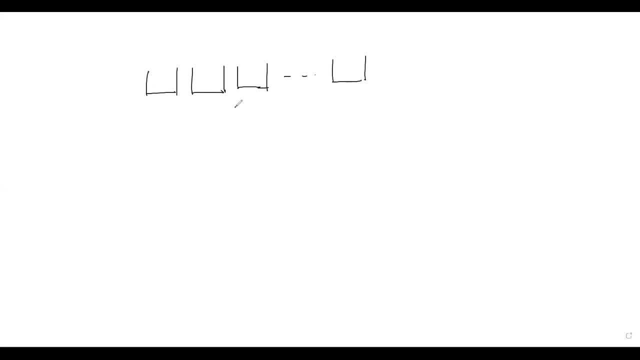 So I have r-boxes here. Now I have n-balls here, so I will say that A1, or, let's see, maybe we will say B1,, ball number 1, ball number 2, ball number 3, and da-da-da-da-da-da to the ball number n here, right? 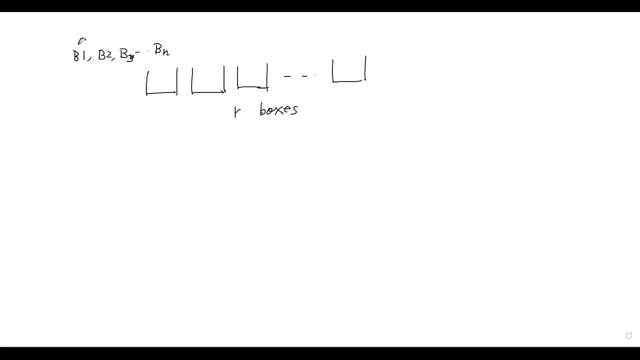 So if they are all Indistinguishable, they are different, right? So how many ways I can distribute to this box here So I can say, oh okay, so for the ball number 1, they have r-chances, right. 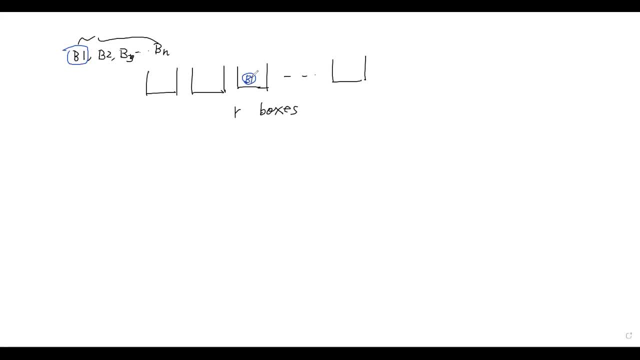 So I can throw the ball number 1s here. So the ball number 1 have r different situation. I can put the ball number 1.. So then the same for ball number 2s here, So I can throw the ball into any. 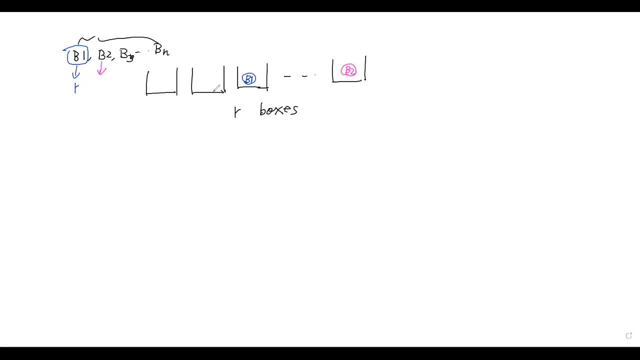 Okay, So I have r-boxes here, so this is ball number 2, so also have r different situations you can throw. So now let's take a look at ball number 3s here. the same way I can throw, so maybe the ball number 3 will be in here, right? 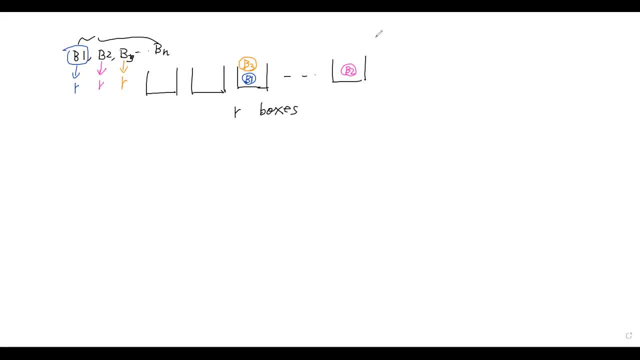 So each ball I will have how many different situations I have r position for them, right? So the total for the question number 1s here is how many ways I can distribute it. Okay, Okay, So what is the total way? 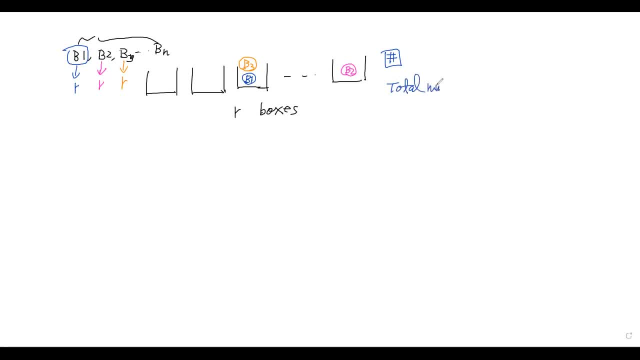 So total number of the way. So how many is here? It's r to the. how many balls here? r to the ns, right? So that is the first ones here, if the balls are distinguished. So that easy, Okay. So this is the first part. 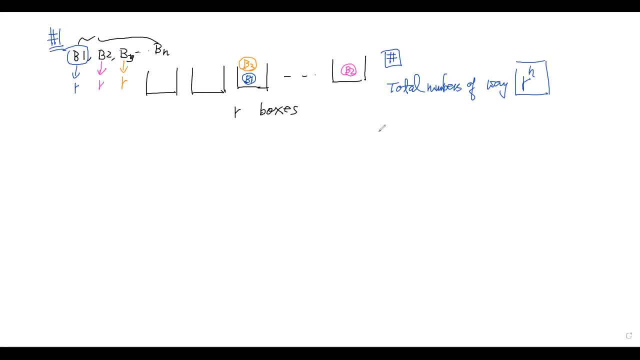 Okay, Now the second part. they said I still have r-boxes here, but then my balls here are indistinguishable, So they are all the same, see here. So instead of using ball number 1,, ball number 2, let's I will say, okay, all these are the balls. here is a, a, a, a, a, a, da, da, da, da da. 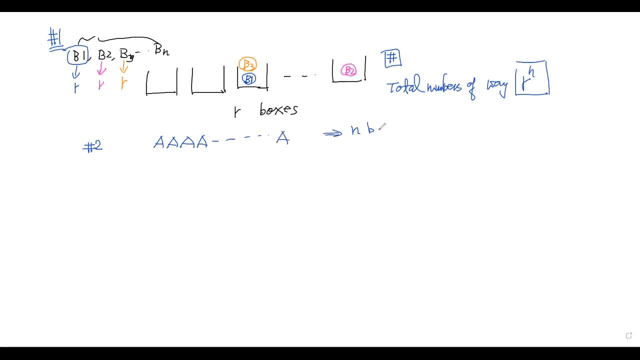 Okay, So those are the n-balls here, right? So they are directly the same I'm going to put into the boxes here. Here, I want to introduce a kind of a concept here. So when you distribute it To the box, it's really, it's similar, like because they are all the same, right? 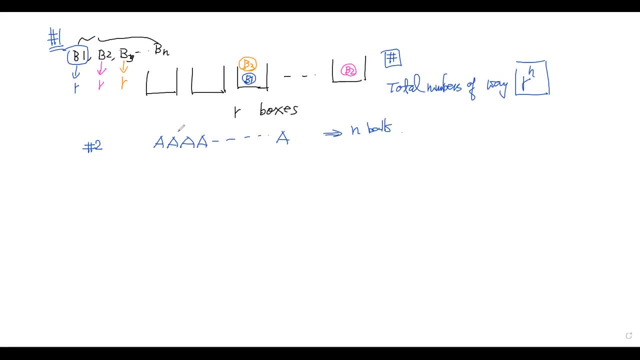 So it's similar, like you just partition that. So you will say, okay, I put it here, put the line here. So this will be my first box. This is my second box here. Then let me put a little bit more a here, right? 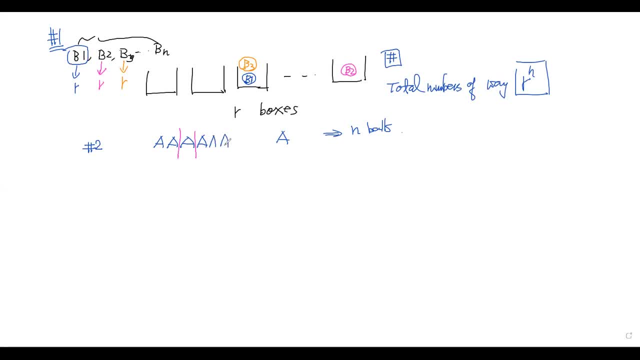 So here. so like this is my a, a, a, so all the different, right. So then you can say: okay, So this is my third box and the fourth box here. So, like me, here there's no partitions layer. 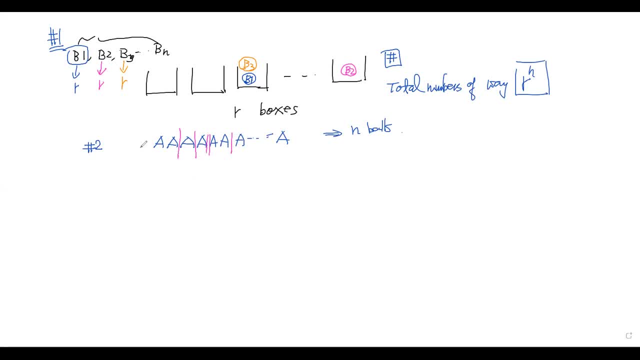 So here is another way I partition that. this strings here, So you can treat this: boxes here, right. So let me this: how do you, you know, do you practice, you know, you, you separate the? this is like the box ones, right here. 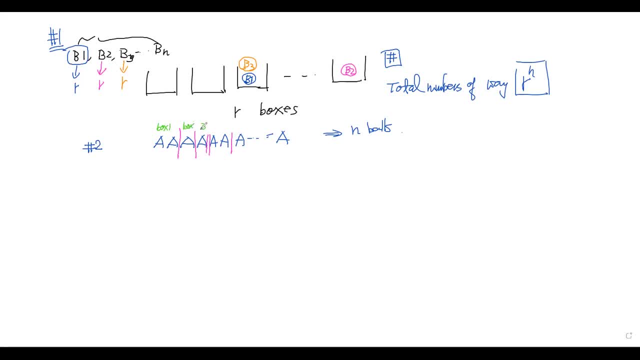 This is a box twos here. This is a box three, box four, five. So it's kind of like a you you just simply do a partition, see here. Okay, So if you understand this concept, then you know. you know if I have a, so if I have the R boxes here, how many loads of partition I have. I have a, what I have, R minus ones here, right? 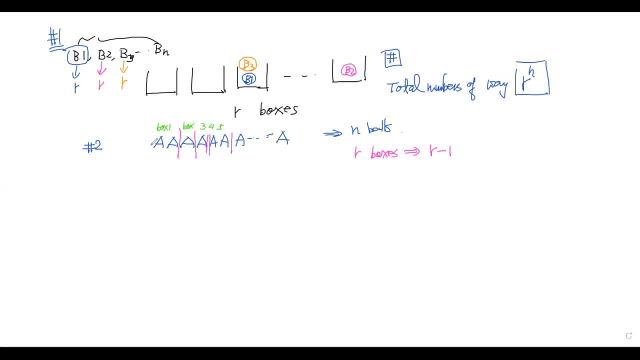 Because you are trying to divide the things to R parts. So it's a very simple. If you kind of say, here I have a, you know I have some numbers here, right, So you want to divide us, let's say here, if you want to divide the number into a, four parts, one, two, three, 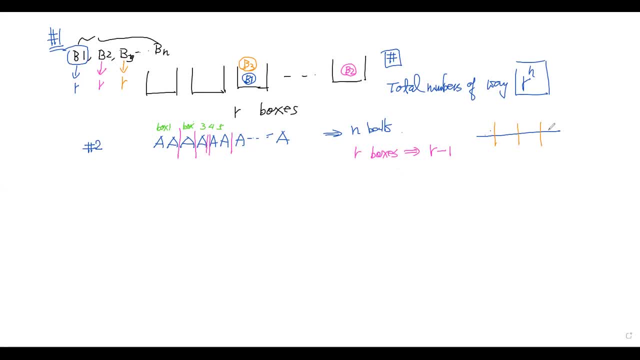 So you need to how many lines here? you need to three lines, right? So if you want to divide the line into a seven parts, here let's say the seven parts. So it's a one, two, three, four, five, six, right? 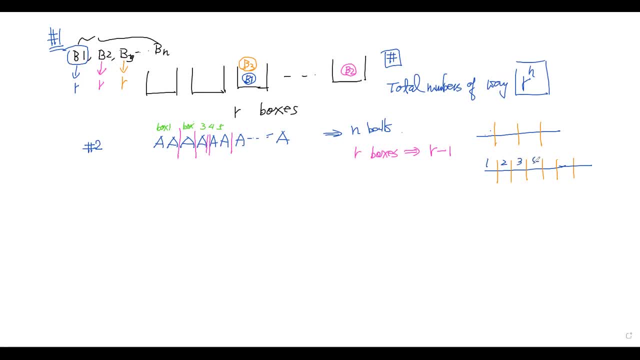 So Because this is a one, two, three, four, five, six, seven, So you divided this line into a seven. So for the R boxes here, so how many loads line I need is R minus ones here. So you treat this things, the whole things is like a whole string. 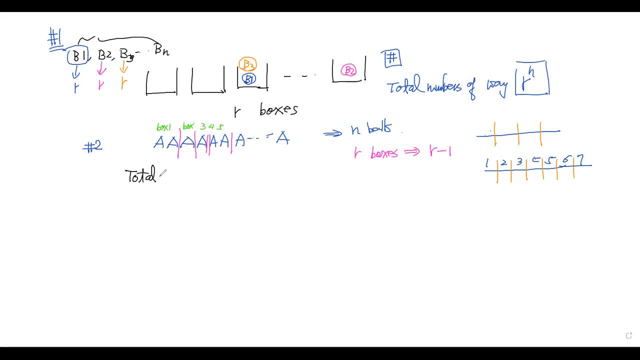 So total, how many elements here I have? Total, How many elements Are here? Here I have: okay, I have an N bar loads of A's here I have an N plus how many loads of bar? here I have R minus one right. 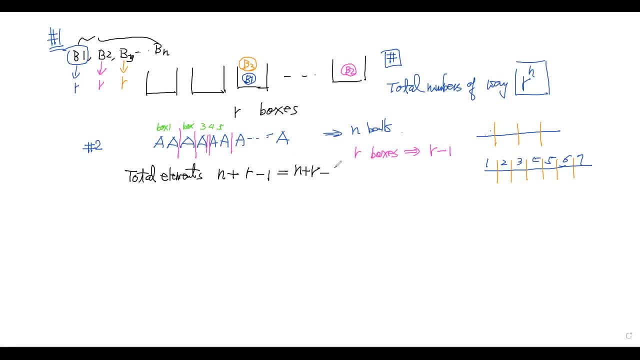 So the total elements I have are N plus R minus one. So the R minus one is how many loads of separation? right, The partition bars I have here, right. So use the concept. If you want to divide it to a four parts- one, two, three, four- then you need a three line. 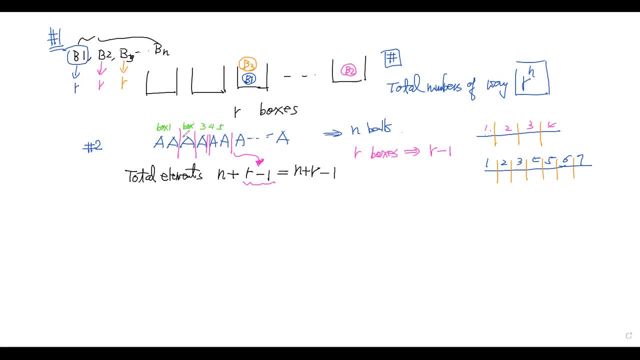 So you divide it. So just same thing here. If I want to separate it into R boxes, here I use R, minus ones here, All right. So now the problem. they ask here they say total. how many different ways here, right? 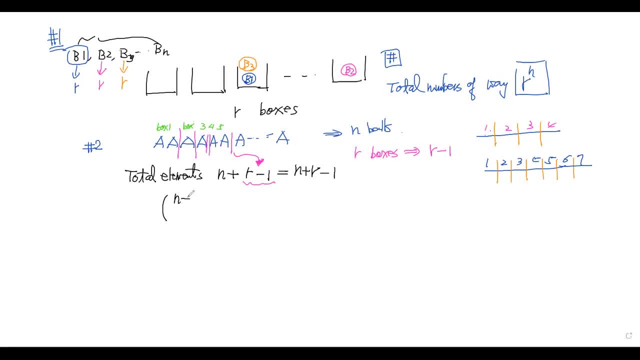 So how many different ways? here We have N plus R minus one, right. Then you want to put this N bars here. So you are At this elements. you want to take Ns here. That is a total. how many ways you can have you get that right. 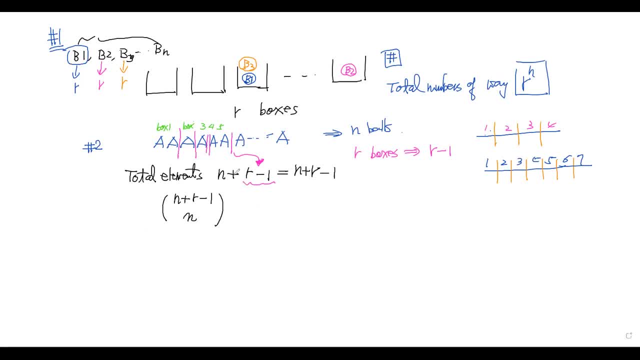 So that's why that means the total. this is a total. how many ways you can, you know, separate or distributed the bar you know into the R boxes here. Okay, So the number three here. let's see here. 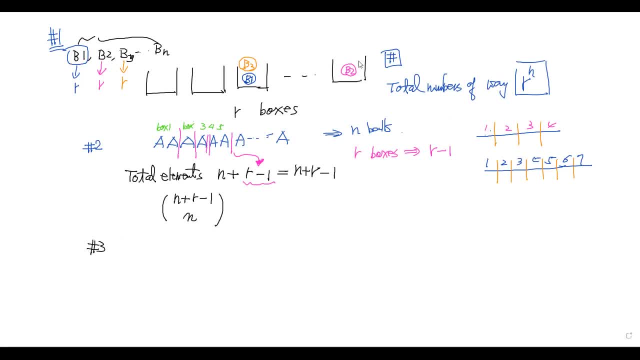 Number three. They said number three, we'll get one more condition. So they said: how about no box? No box can be empty. Okay, Think about, if no box can be empty, what's that mean? That means for each box. here I need to at least put what. 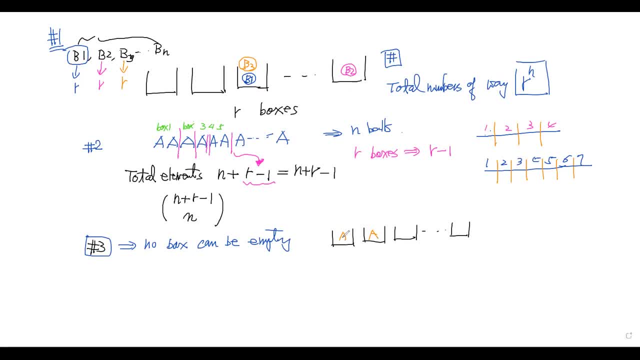 At least have The one ball, my A ball, here, right? So at least I'm going to have one box of one box here, So that's why I can make sure no box will be empty. So after you do that, how many balls left? 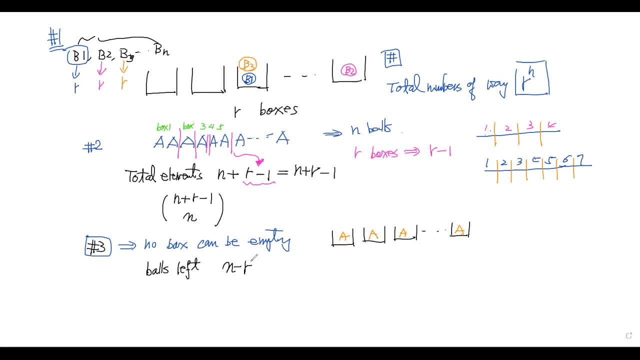 How many balls left here? You have N minus R balls left, right. Okay, Now for this N minus R ball. then you can distribute it to the R box again, So you will have A, A, A, da, da, da, da, A, A, something like that, right? 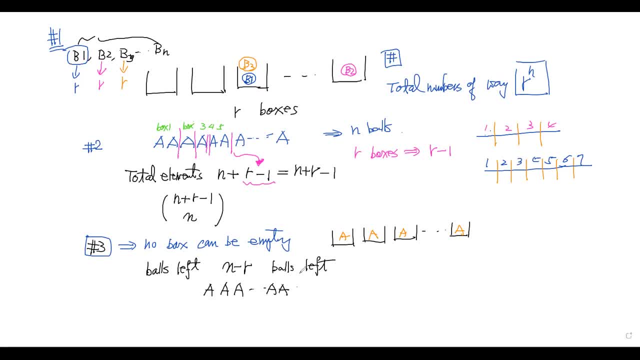 So now you are distributed. So total here- be careful, see here right. So total here. you only have N minus R balls here. Okay, Then you distribute it into the R box. So it's still the one. So you can do like this: do the partition. 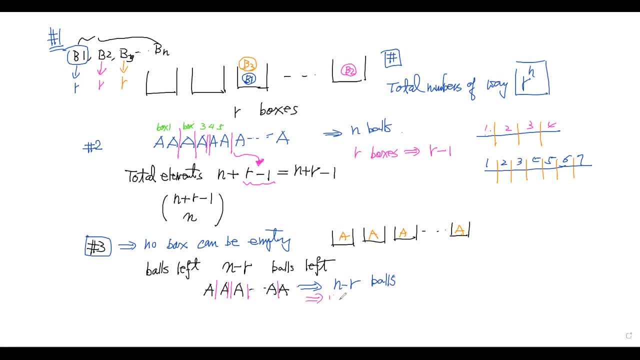 So how many of those bars we have here Still, how many R minus one, right, Because the remaining I can distribute to the R boxes here. So I want to kind of partition into R parts. So I need to use R minus one, those you know, those bars here, right? 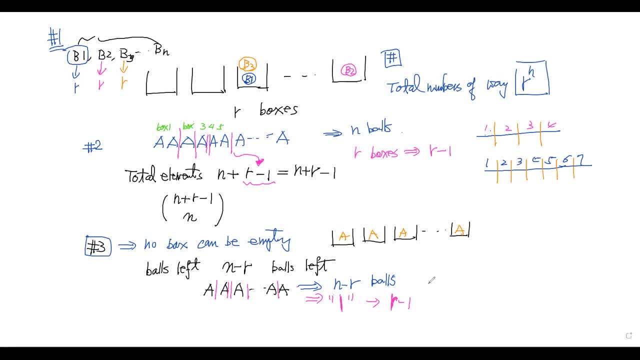 So that's what the those bars here I have R minus one. Okay, So now let's take a look. So what is my total elements right now We have? we have how many I have N minus R plus R minus one, correct.